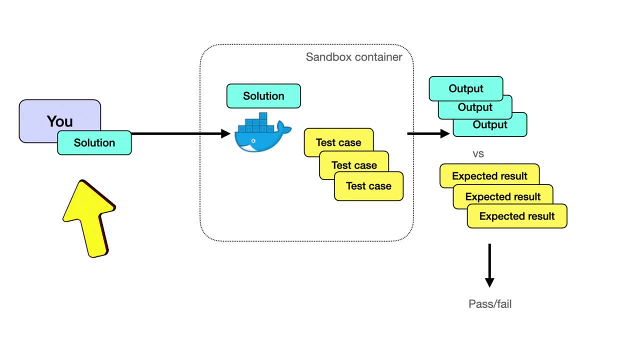 their code, a whole process is set into motion. The backend code of these platforms springs into action and spins up something known as a docker container. Think of it as a sealed-off sandbox environment where your code can play freely without affecting or being affected. 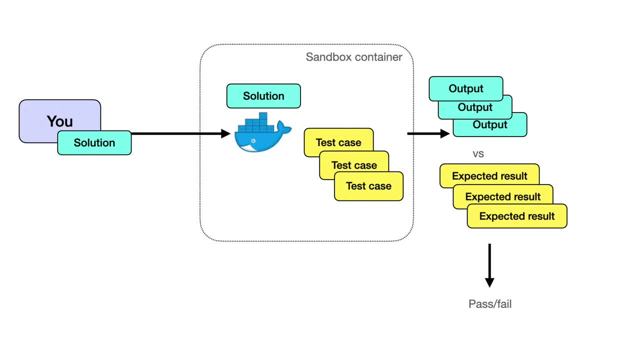 by the host environment. Now, within this safe little sandbox, each of your test cases is run. Your code is executed inside the container, with each test case being fed as input. The output of your code is written to a local file. The platform then takes this output and 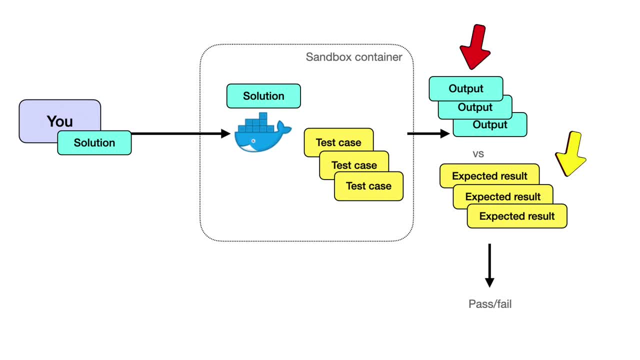 compares it to the expected output. If the results of all the cases match the expected output, then you're in luck: Your code gets the green signal and is accepted. But what happens if your code takes too long? Well, that's where we have the concept of a timeout. 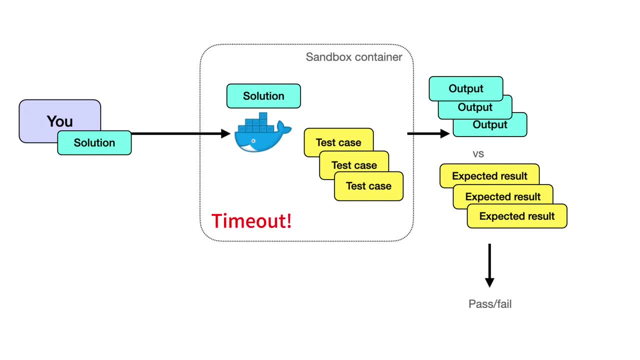 Each of these containers has a specific timeout duration. If your code keeps running and running without a sign of stopping, eventually the containers will be shut down and you will get a TLE on the front end. Now you might be wondering: why are we talking about all this? 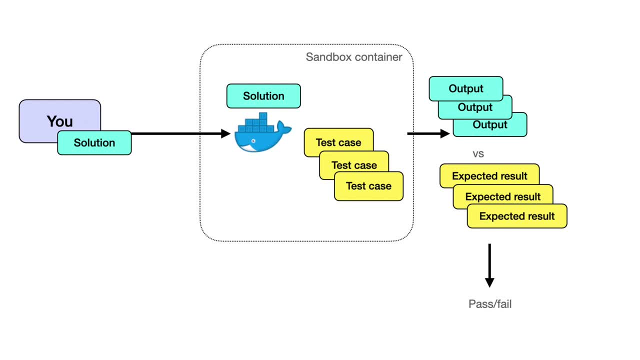 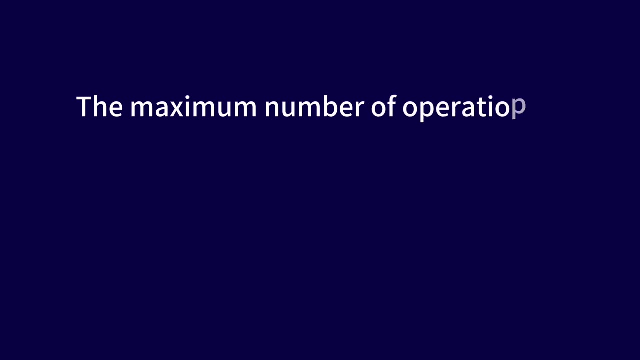 Because this is where the constraints in your problem description come into play. These constraints are not arbitrary. They have a real impact on whether your code runs successfully within the timeout. Based on our collective experiences and many hours spent solving problems, we've noted that the maximum number of operations generally allowed before hitting a timeout is: 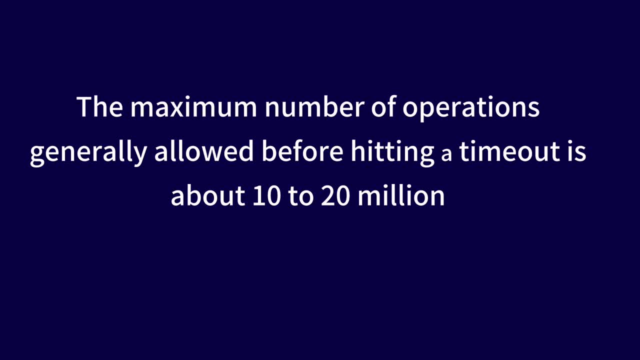 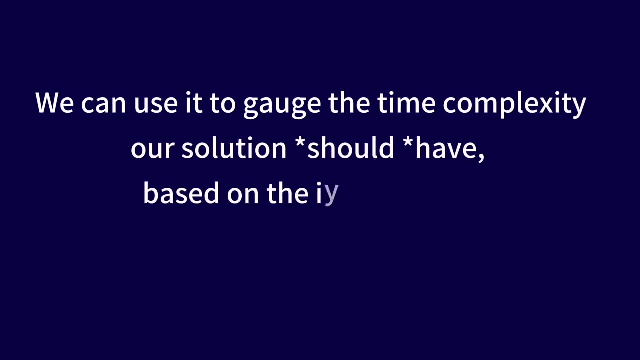 about 10 to 20 million. Now, that's a significant number, but how do we make use of it? We can use it to gauge the time complexity our solution should have, based on the input size or N. Let me break it down for you: IFN is less than 20.. 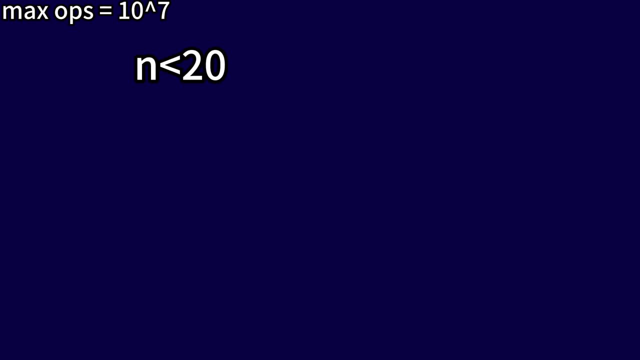 With such a small input size, we have a lot of room to work with. We can typically afford to use root-force solutions here. Why? Let's do the math: 2 to the power of 20 equals 1 million, which is well within our maximum operation limit. IFN is up to 3,000.. With this range, 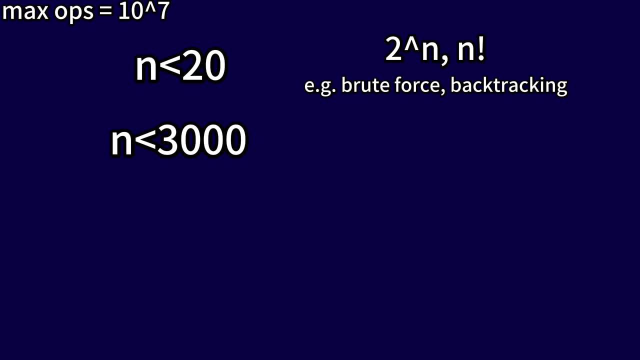 we're starting to push the boundaries a bit and will need to be a little more careful. An algorithm with a time complexity of O is usually the best fit here. An N-squared operation for 3,000 still falls within our limit of 20 million operations. IFN is between 3,000 and.